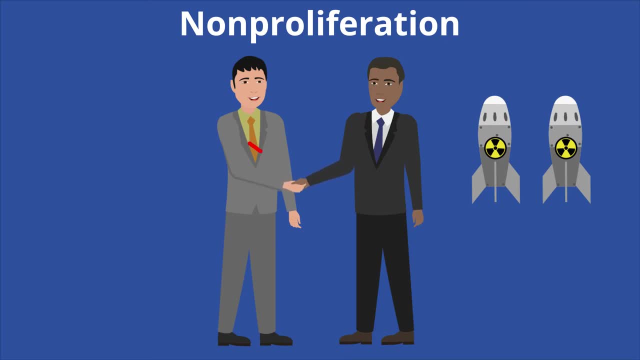 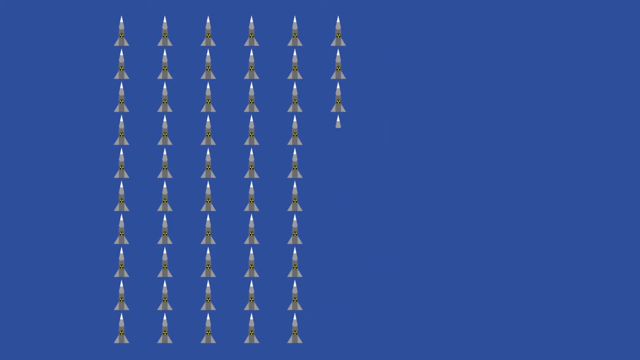 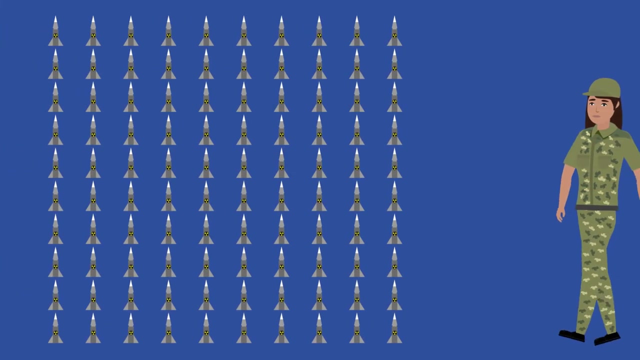 peacefully. Nuclear states will not assist non-nuclear states in acquiring nuclear weapons in any way. Second, disarmament: The article regarding disarmament vaguely states that nuclear states should move towards general disarmament of nuclear weapons. However, this aspect of the treaty is criticized for its lack of precision, allowing nuclear states to 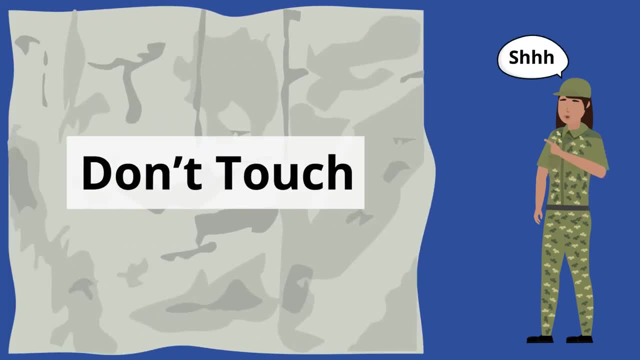 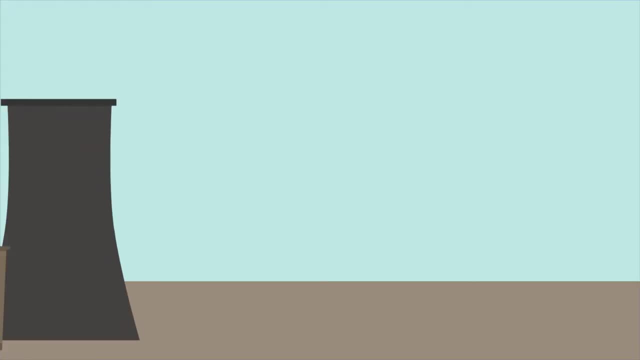 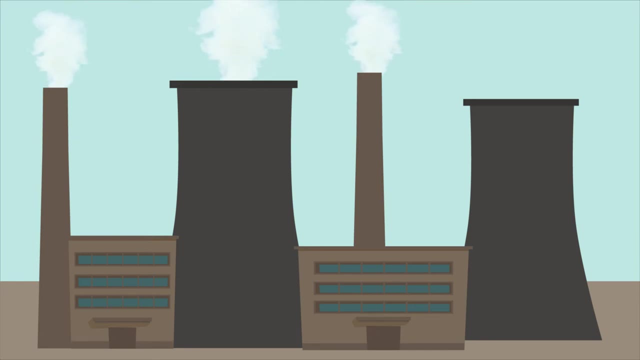 maintain their nuclear arsenal. The five nuclear states in this treaty have failed to effectively move towards disarmament, which has sparked controversy over whether non-nuclear states should uphold their end. Peaceful use of nuclear technology: The treaty recognizes the right of all nations to develop nuclear technology for peaceful purposes, such as providing electricity. 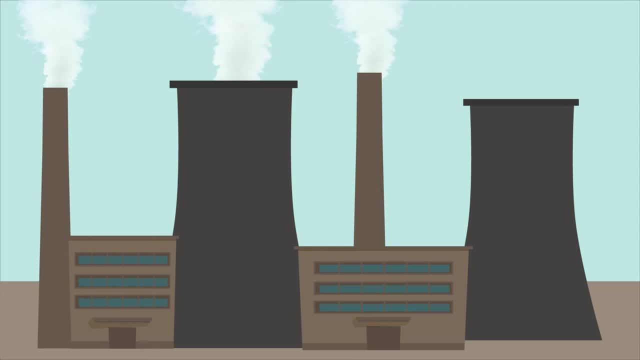 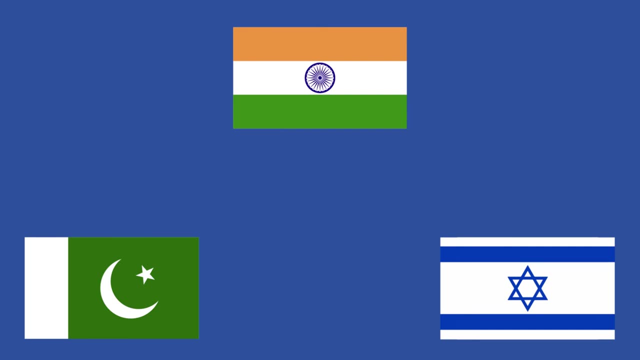 and energy, and demands that non-nuclear states get assistance in their efforts to develop nuclear technology. Although this treaty currently has 191 signatories, a few nations with nuclear weapons have not yet signed the treaty, including India, Pakistan and Israel, whose possession of nuclear weapons has not been proven yet. 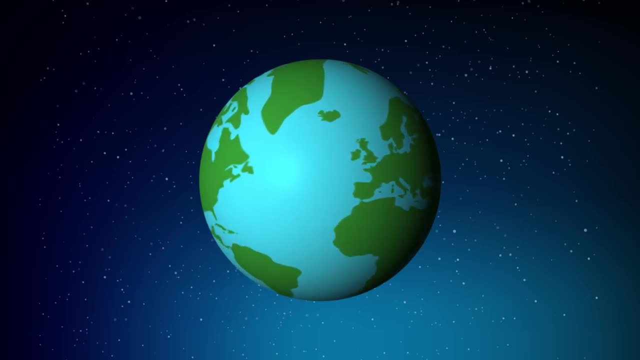 Because some nuclear states have not signed the treaty, there is concern around the treaty's effectiveness. However, the non-proliferation treaty remains the most significant global effort to eliminate the spread of nuclear weapons. The amount of nuclear weapons in the world today are: 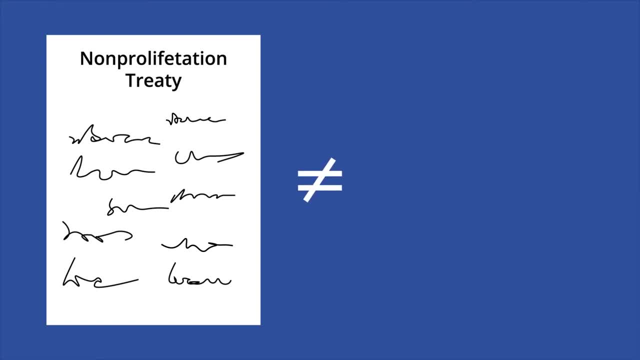 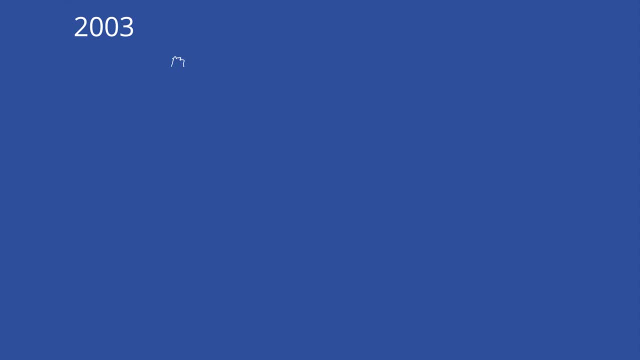 only one-fifth of what they were when the NPT was signed. However, nations who have signed the NPT, as well as those who have not, continue to engage in behavior that is contrary to the goals of non-proliferation. In 2003,, North Korea decided to withdraw from the non-proliferation. 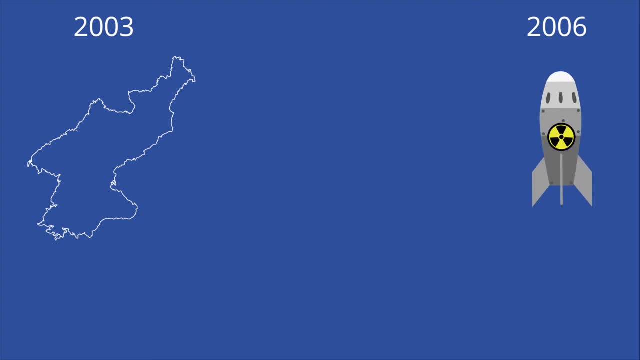 treaty and three years later, the North Korean government tested its first nuclear weapon. Recently, there has been concern that Iran is also seeking enough nuclear power to create a nuclear weapon and may also choose to withdraw from the NPT in order to do so In 2015,. Iran and six other 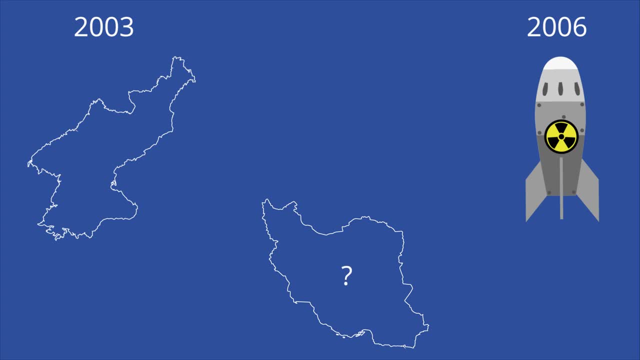 nations reached an agreement to restrict its ability to build a nuclear weapon in what is known as the Iran Nuclear Deal. However, the United States' withdrawal dramatically weakened the agreement and eventually led Iran to withdraw as well. The United States and Russia account for 90% of the nuclear weapons on Earth. 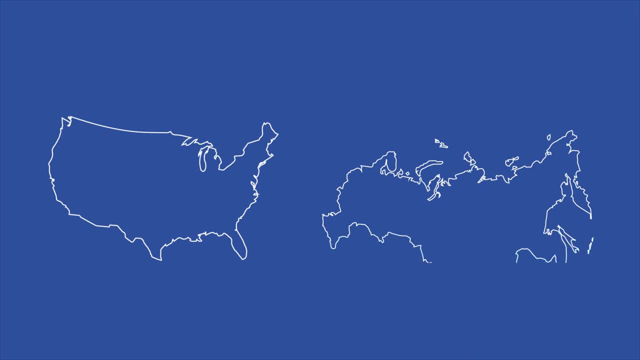 While the amount of active weapons held by these countries has drastically reduced since the end of the Cold War, both continue to modernize their nuclear arsenals. Likewise, tensions between the US, Russia and China have risen in recent years, making the goal of complete nuclear disarmament.